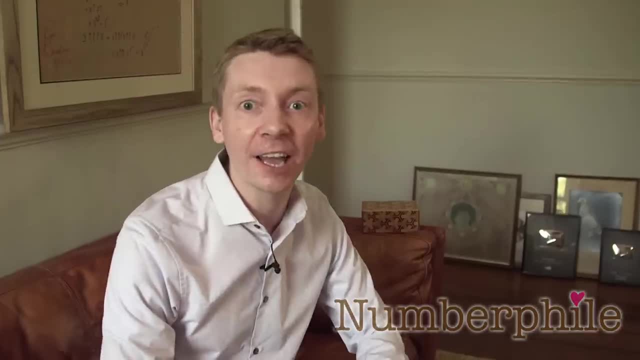 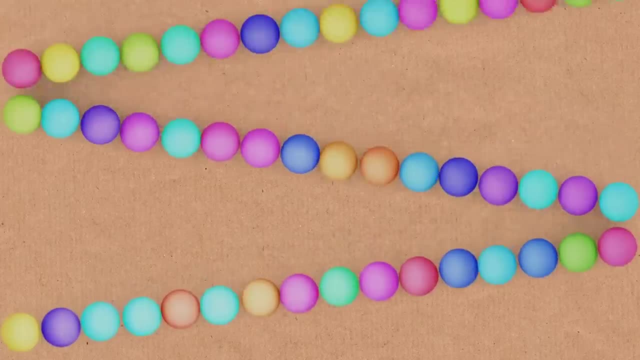 We're going to talk about a classic problem in mathematics. This problem is 400 years old. It's about sphere packing. The question is: what is the best way to pack spheres, And by best I mean what is the densest way of packing spheres. And it's thought that the best way of packing 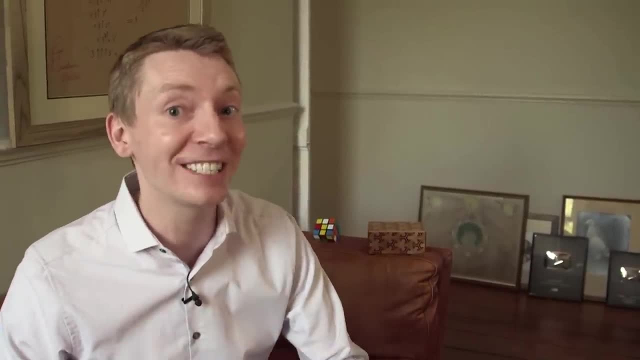 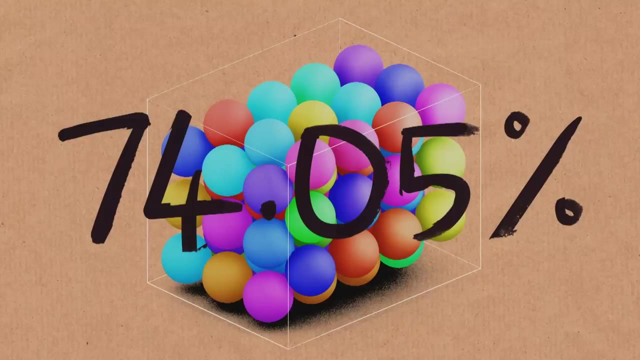 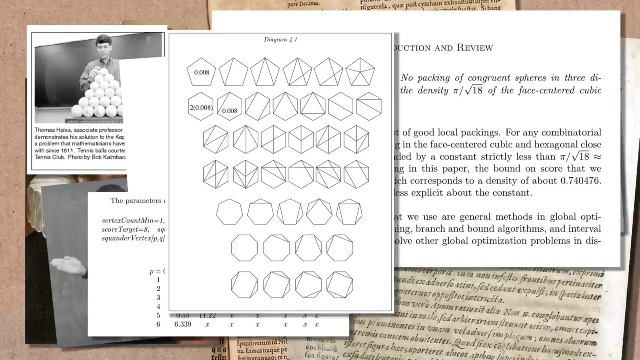 spheres is 74.05%. So if you were packing a container it would be 74% full. Now it's been thought that that is the best way of packing spheres for 400 years and it was finally proven in the 1990s. However, the referees, when they looked through the proof, thought they were 99%. 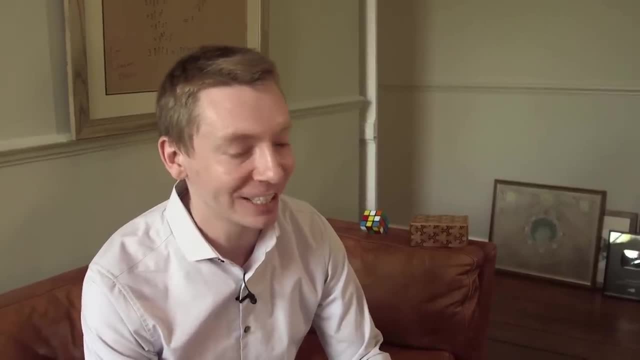 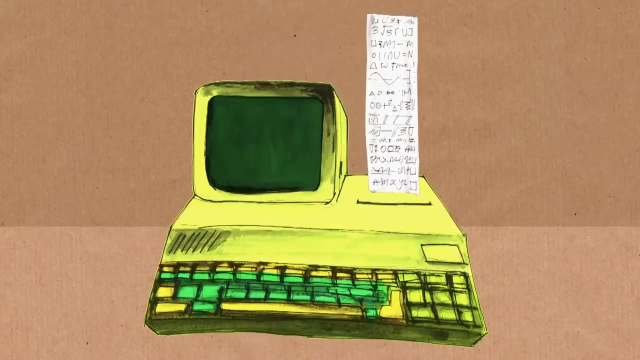 certain that the proof was right, So that's kind of slightly unsatisfying. So then they started a 15-year project to really make sure that this is correct. They've rewritten the proof in very formal mathematical language which allows a computer to automatically check the proof. 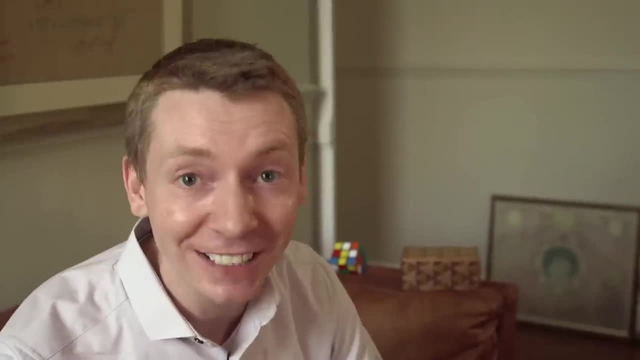 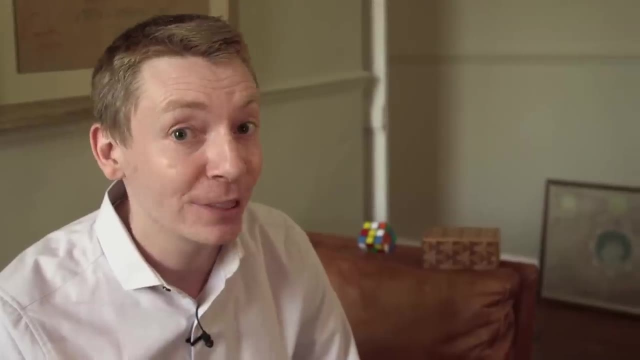 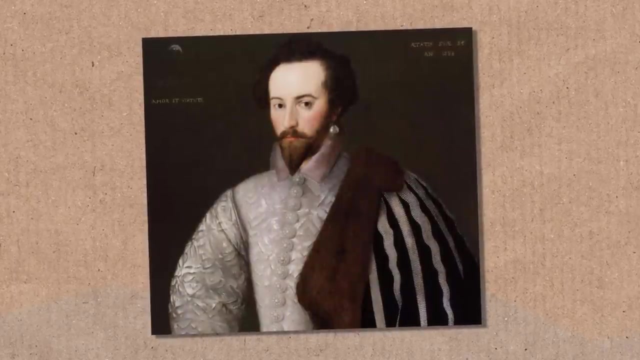 Which was finally accepted in 2017.. Finally proving the conjecture about how densely you can pack spheres. But the problem itself goes back to Sir Walter Raleigh. of all people, Sir Walter Raleigh is very famous in Britain, but he's an explorer. He's the guy who put his coat over a puddle, so 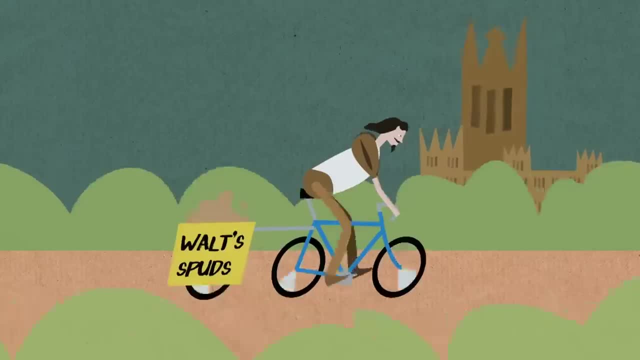 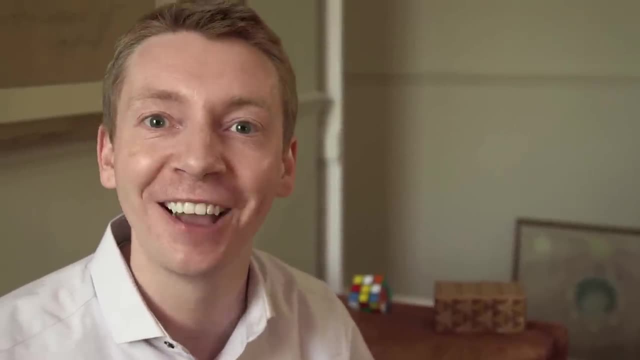 Elizabeth, I could walk over a puddle. He invented the potato and other lies- Very famous in Britain, I know- And he wanted to know the best way of packing his cannonballs on his ships. So he asked his mathematician, because everyone should have a mathematician. 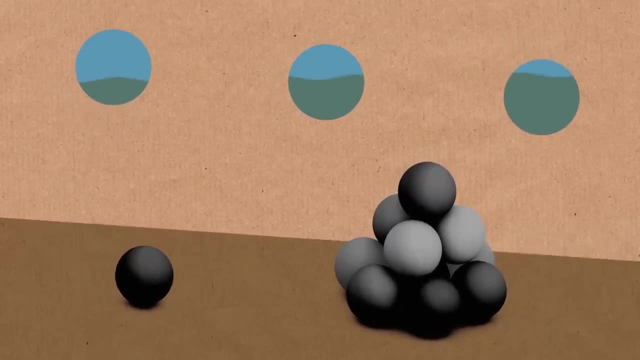 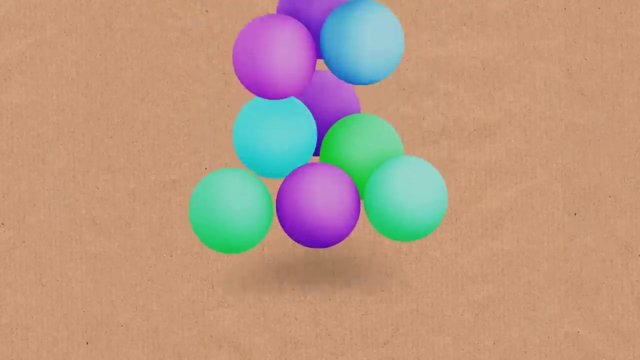 a guy called Thomas Harriot, And so he started looking into the best ways of packing cannonballs. So perhaps one of the obvious ways of packing spheres would be something like this, which is a pyramid shape, Well, with a triangle base, So a tetrahedron. You see people stacking. 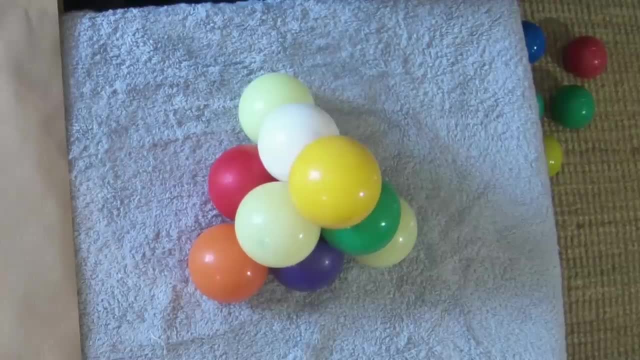 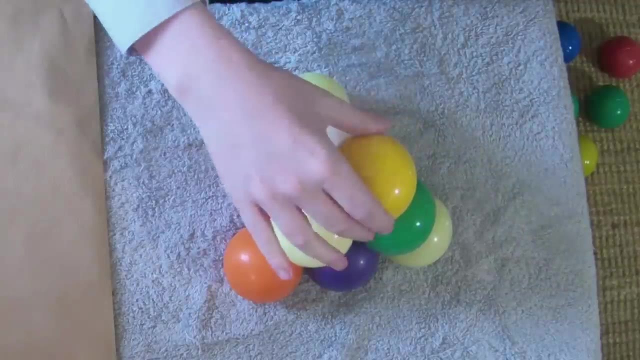 oranges or something in the supermarket. That would be one way of doing it, But another obvious way of packing spheres would be a square base pyramid. Let's try that. So let's try that. instead Break this apart, Let's try and make a square base pyramid. Let's do a couple of extras. 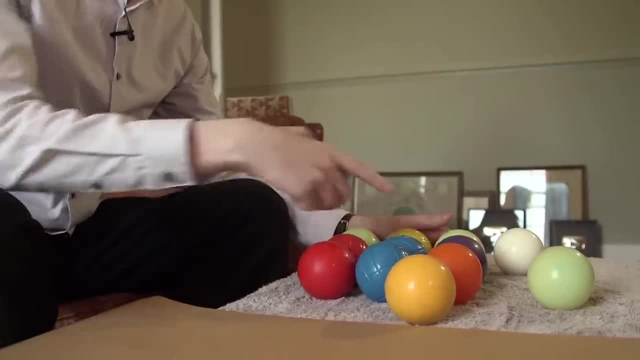 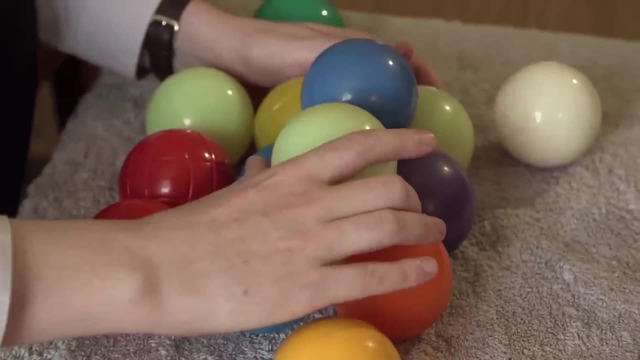 Here we go. Now it's obvious where to fill the next layer, because we're going to fill these dimples here. So let's do that, So we can fill these holes with our next layer of spheres. So I'm going to put that one there, Let's put this one here. Let's put this one here. 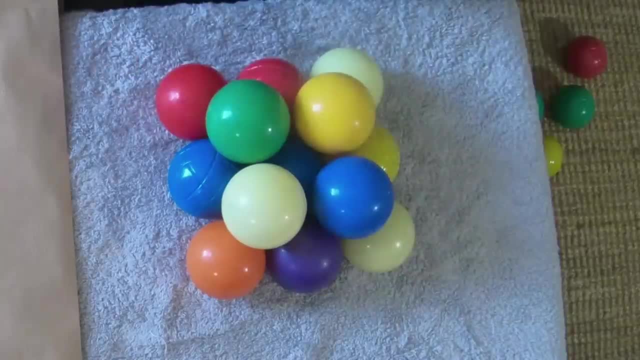 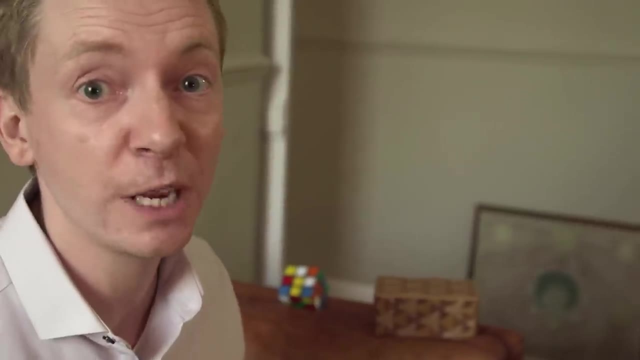 And if we're lucky, we should be able to crown this with our last one, like that. So we get a square pyramid. So that's another way of doing it. Perhaps another obvious one would be with a hexagonal base. So we're going to look at that too. So let's try and make a hexagonal base. So 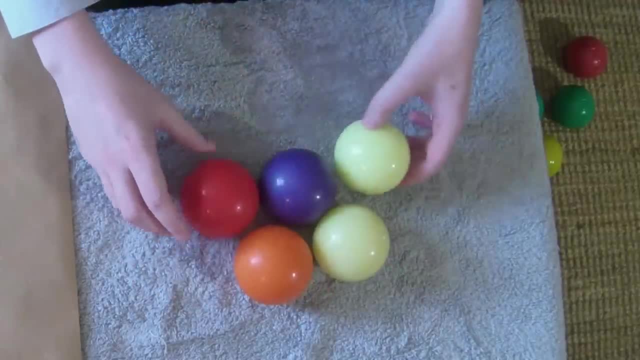 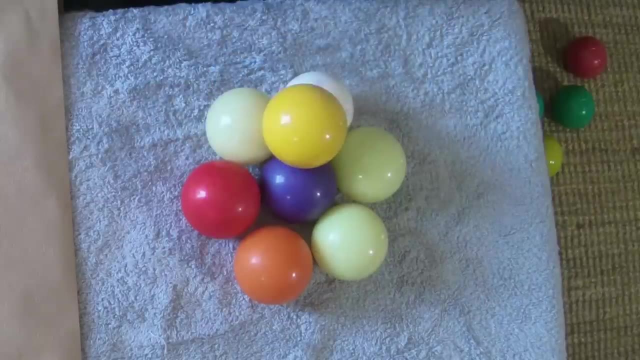 we have a central one there. Let's make a hexagon around the center And then for the next layer we would fill in those obvious dimples. So there'll be one there, perhaps, And one there perhaps. Let's do one there. 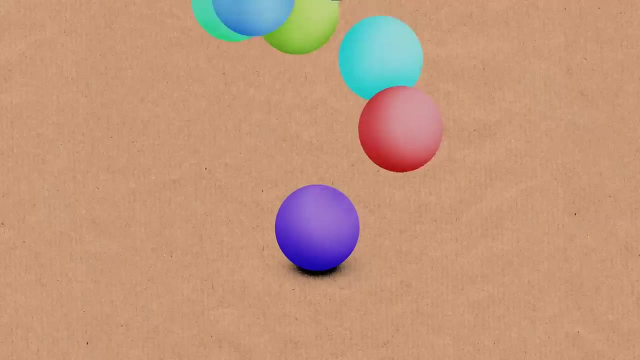 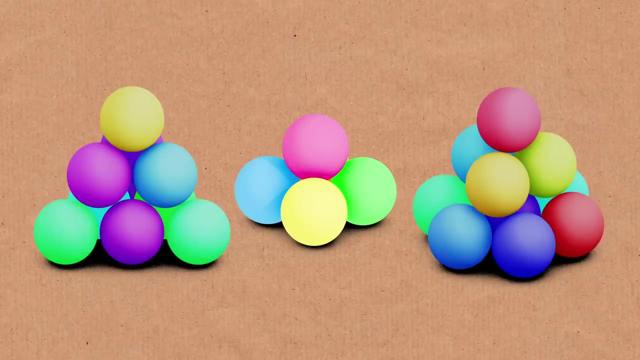 And I could crown this off with another one, But what I wanted to show you- and this is what Thomas Harriot noticed- is that all those packings are actually equivalent. They're all the same And they all have the same density as well, which is going to be this 74.05%, So you might be able to. 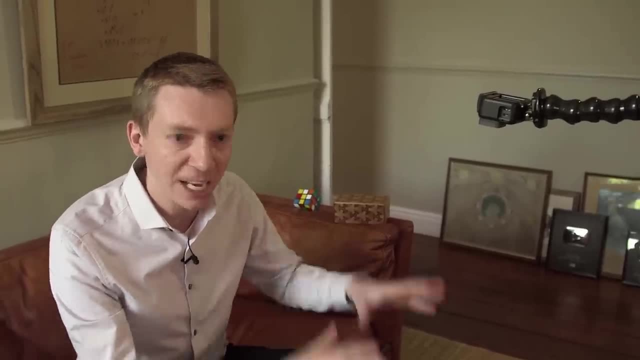 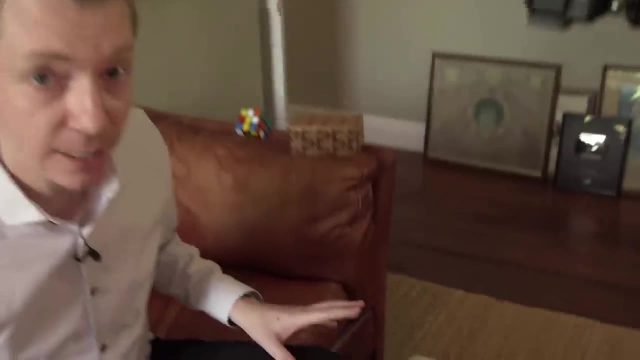 see that the hexagonal packing is the same as the tetrahedron one. It's the same kind of packing, layer by layer, But this is less obvious. I wanted to point out. This is also the same as the square base pyramid, but it's tilted on its side. Look there. Can you see that? 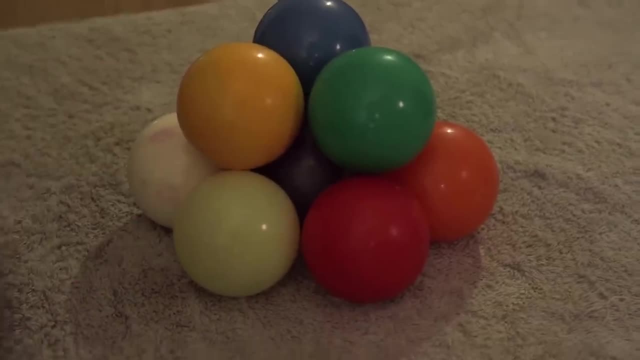 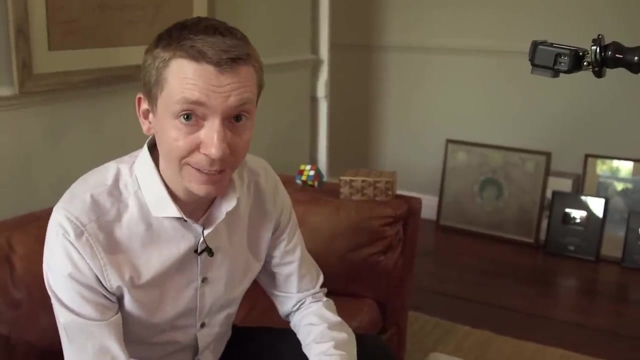 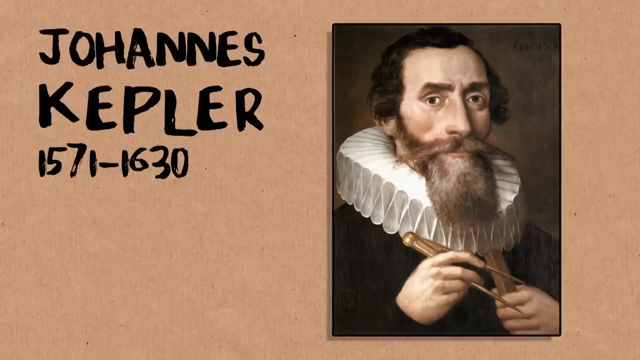 square there. So that square would be the square base of the square based pyramid, but it's just tilted on its side. So all these things are absolutely equivalent. They have the same density, which is 74.05%, Actually Thomas Harriot's pal, which is Johannes Kepler. 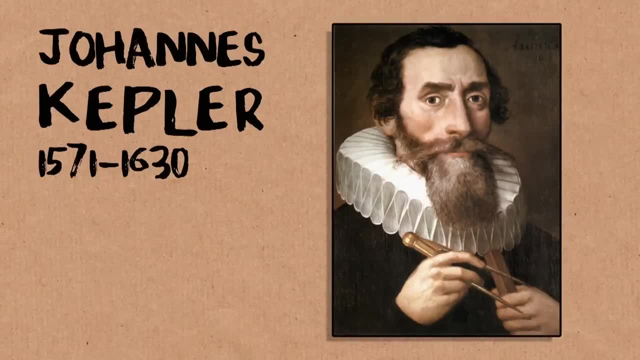 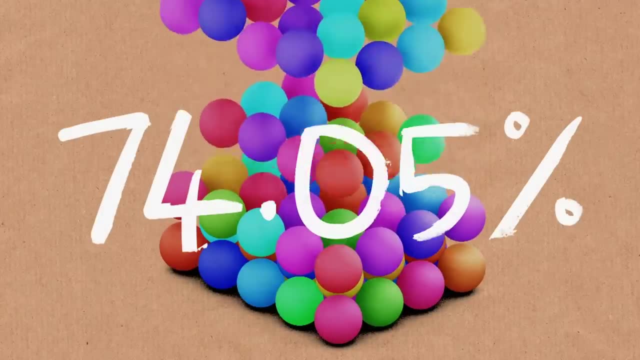 who, you may know, decided that this would probably be the most dense packing possible. So this is now known as Kepler's conjecture that this is the best possible, which is the 74.05% figure. So let's have a look where that figure comes from. Incidentally, this is one of the early 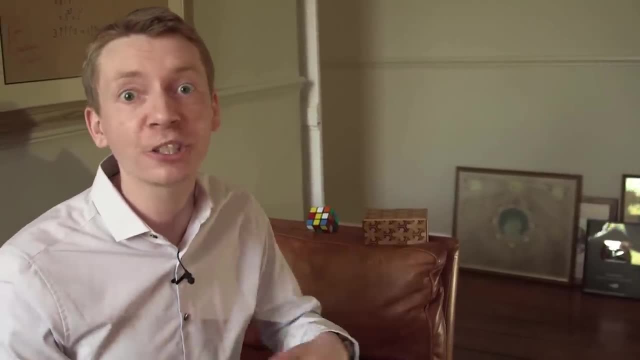 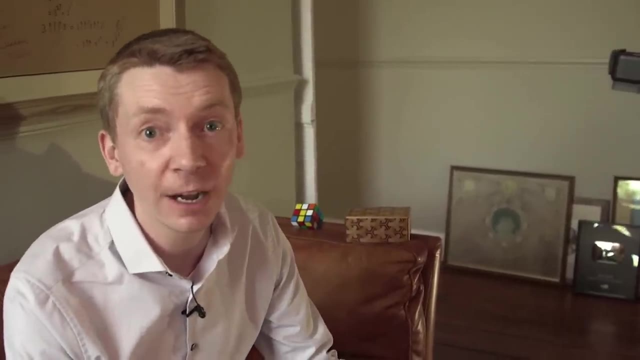 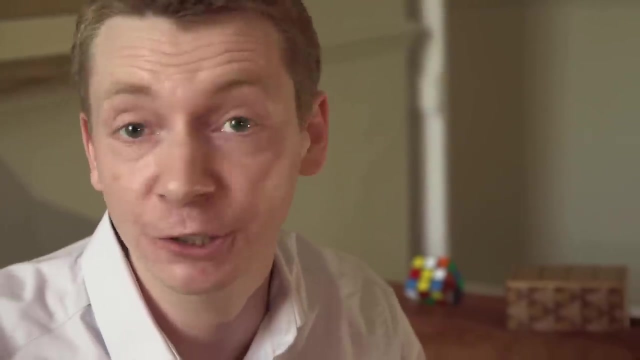 beginnings of how atoms work or how we started to learn the structure of atoms. If these spheres were atoms, then this kind of packing is what you find in I don't know, aluminium or copper- if these were the atoms of copper- or in crystals like just table salt, If you look at a crystal, 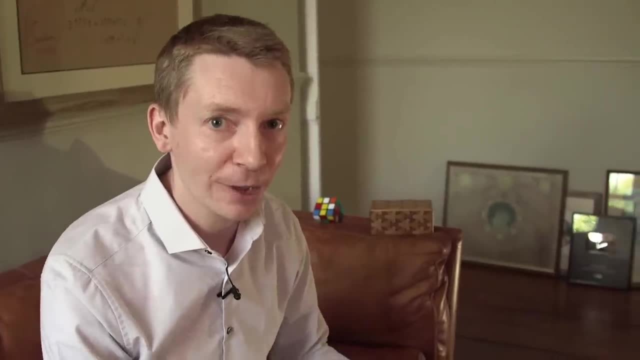 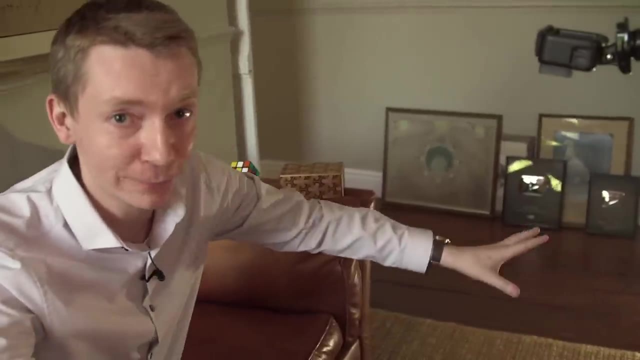 like that. you get this kind of packing. But let's look at where that figure comes from. So here's a small square-based pyramid. Now this just repeats forever. If you just imagine that repeating forever, that would be the idea of packing. What about if we can cut this up into some sort of unit? 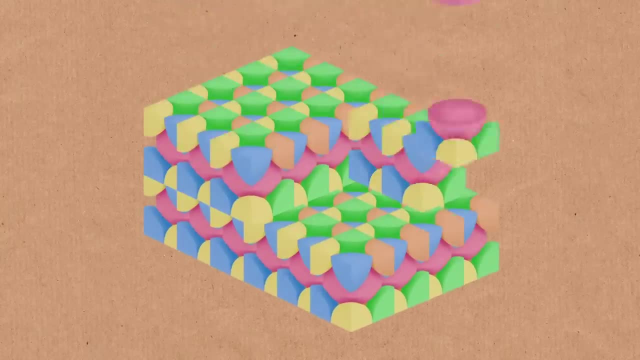 that we can then just repeat. Then, if we work out the density of the unit, that does the whole thing. Okay, let's do that. What I'm going to do is I'm going to slice up this pyramid into a box. I'm 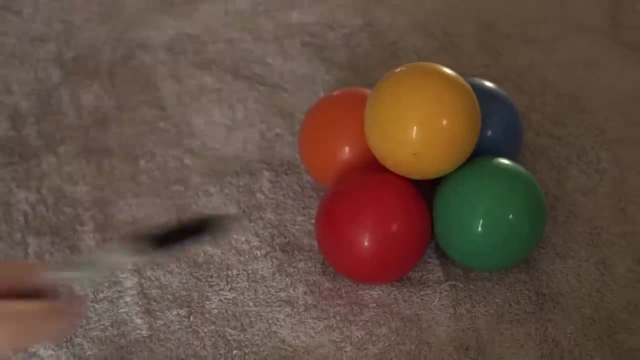 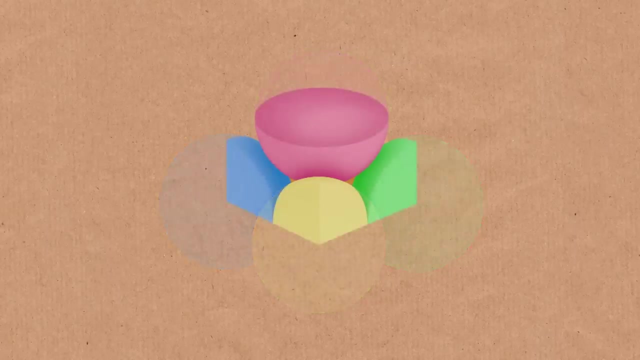 going to cut a horizontal line across the top layer, I'm going to cut a horizontal line across the bottom layer. So I've cut them in half, and now I'm going to cut four vertical lines. So now I've created a box, and that box, if you repeat it, will give you the whole packing. So now I want to know. 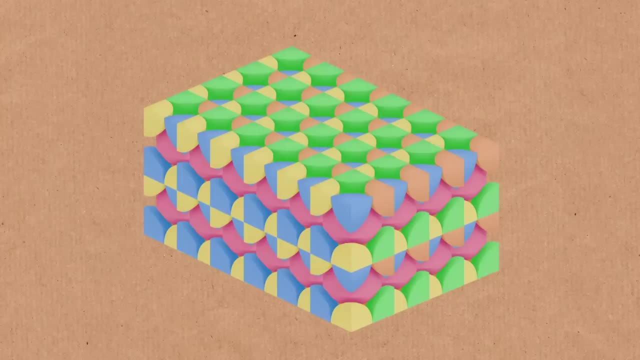 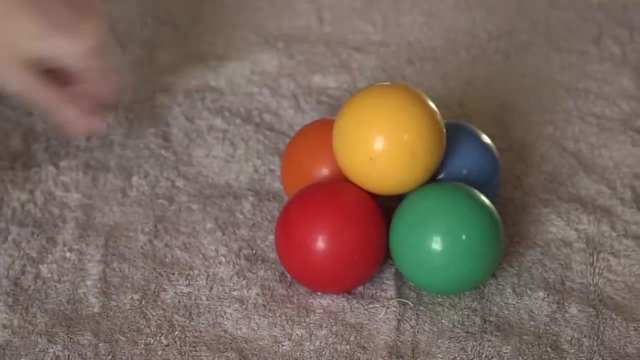 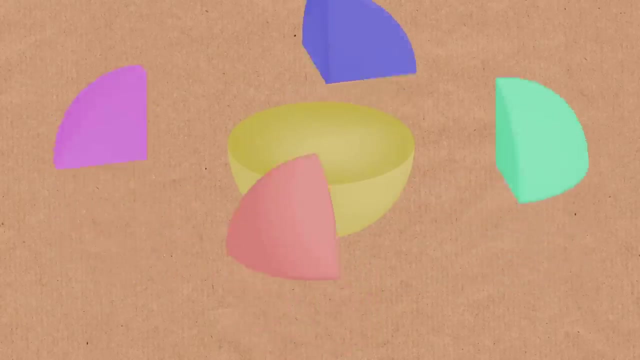 the density of the spheres inside that box. Well, that box contains exactly one sphere. We've got half a sphere from the top and then from the bottom layer. I cut it in half and then I cut it in quarters, So I've got four eighths of a sphere. So all together that would make one complete. 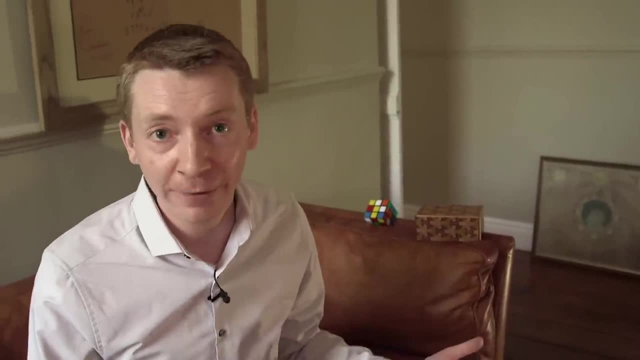 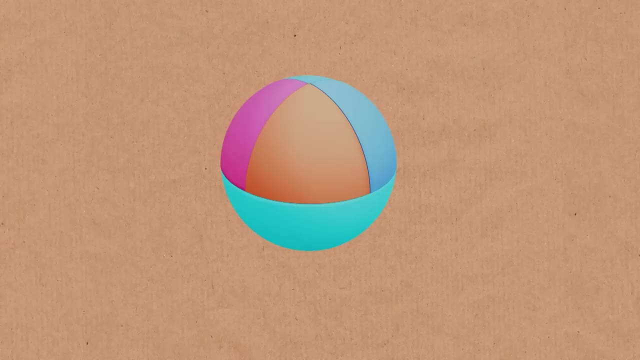 sphere. So what is the volume of one sphere? Well, there's a formula for that. So that is four pi over three. well, r cubed, but let's just say it has radius one, because there's no reason why not. So I'm just going to say it's four pi over three. So that'd be the volume of the. 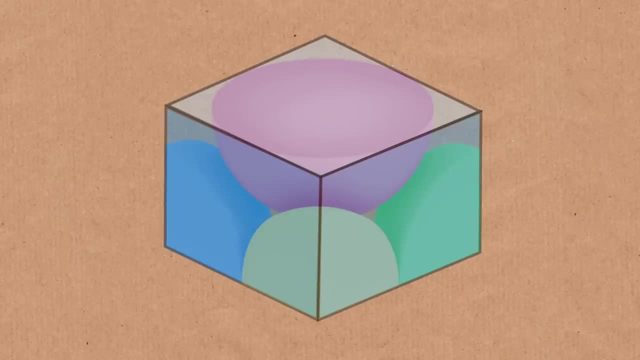 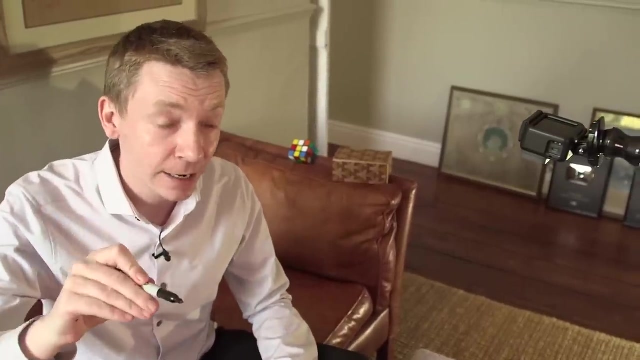 sphere. Now the box that I've made. well, we've cut it across and vertically, and so on. It would have a base of two by two, so it'd be an area of four, and then we could times that by the height. 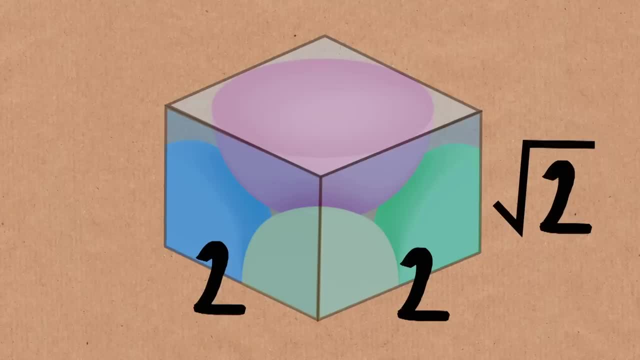 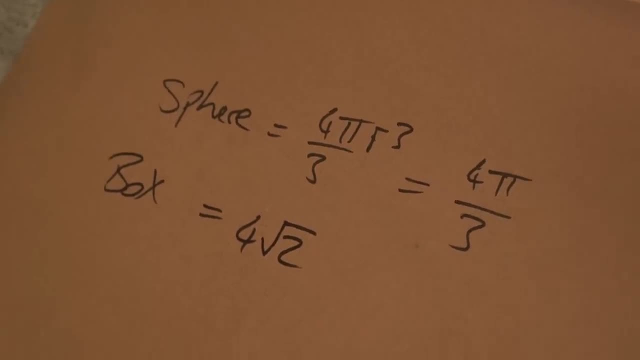 With a bit of Pythagoras you can work out that the height is root two, So the box would have a volume of four root two. So now to find out the density, we're going to divide the volume of the sphere by the volume of the box. 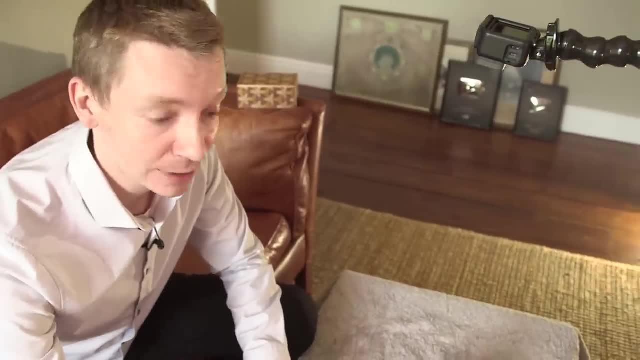 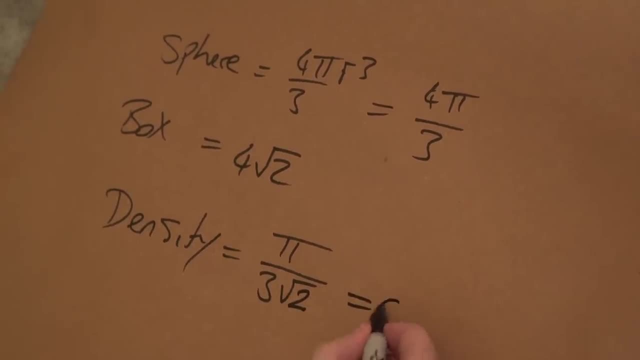 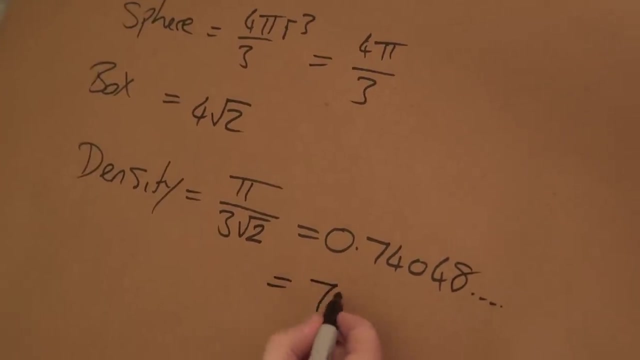 So if we divide through, you might be able to see we're going to get the cancel out here with these fours. The density is going to be pi over three root two and that figure is something like 0.74048 and so on, and that is where our 74.05 percent figure comes from. That is the density. 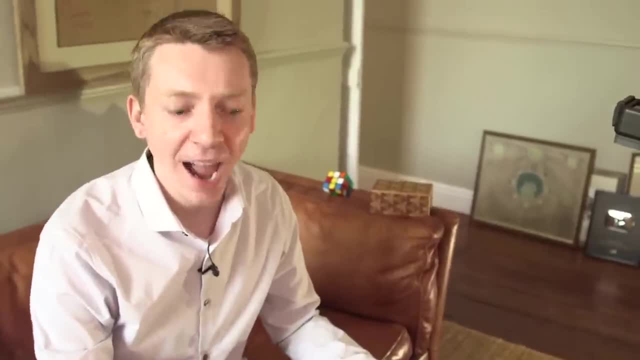 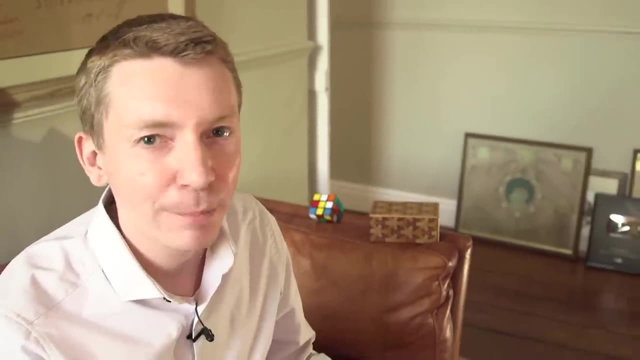 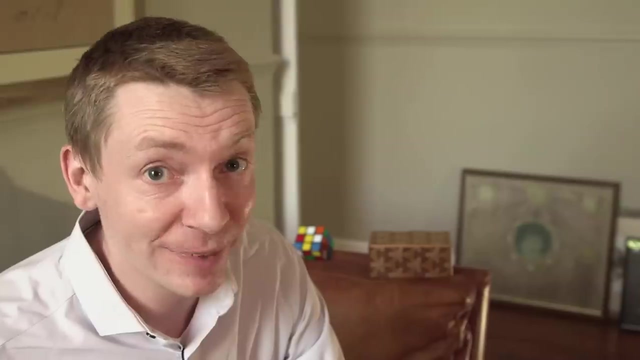 of these obvious packings and it might seem obvious that that would be the best way of doing it. I think so. I think it's obviously the most dense, but proving it's the most dense, that was actually quite difficult. So one of the first people who tried to take on this problem and see 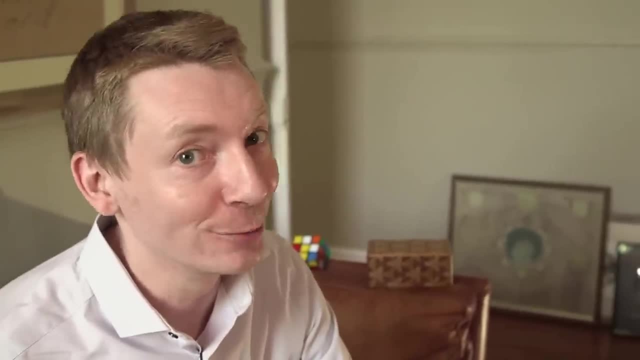 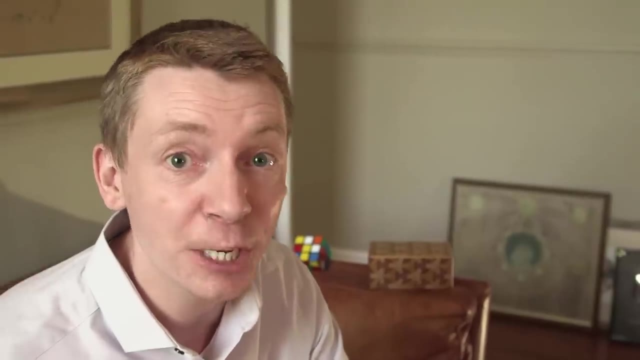 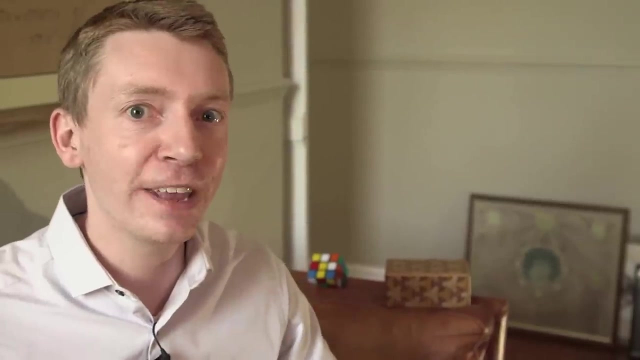 if they could prove that this was the best was Gauss. Gauss, one of our great mathematicians. his name comes up a lot in these things, and what he did show was that this was the best packing, the most dense packing if the structure is regular, But he didn't show if it was always the. 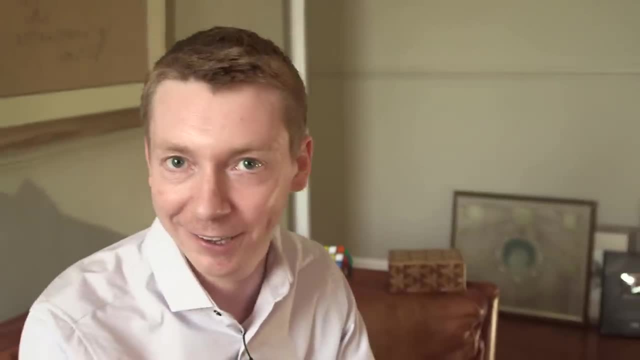 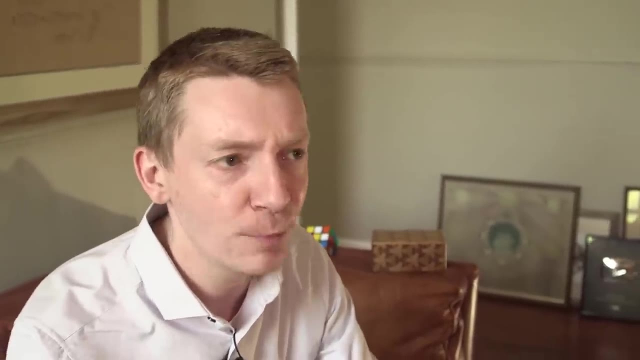 best. So maybe there's an irregular packing that would be better than this. That is possible. So this was still an open problem. It actually became a very famous problem. It became one of David Hilbert's problems, which was a set of problems for 20th century mathematicians. 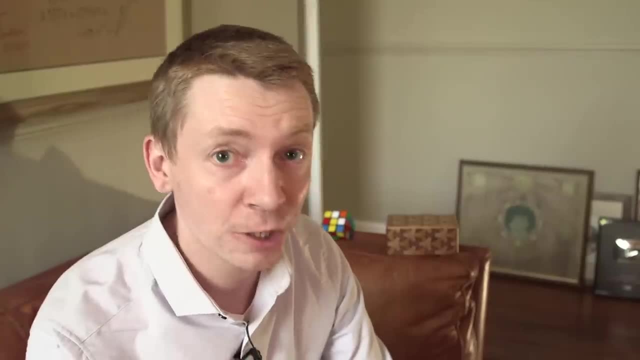 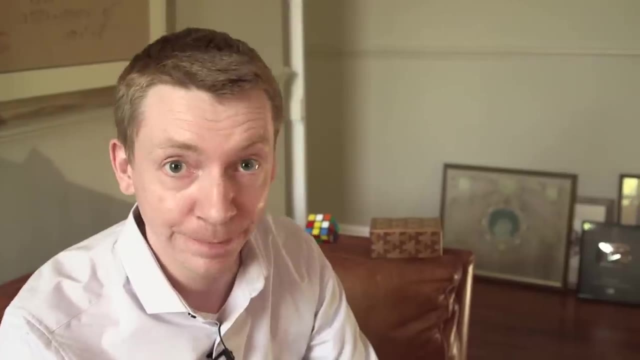 It was his 18th. Eventually, though, it was proven in the 1990s. And what they did is? they slightly changed the way we were thinking about this, So I'm going to try and show you what they did. I'm trying to give you the gist of the idea. It'll 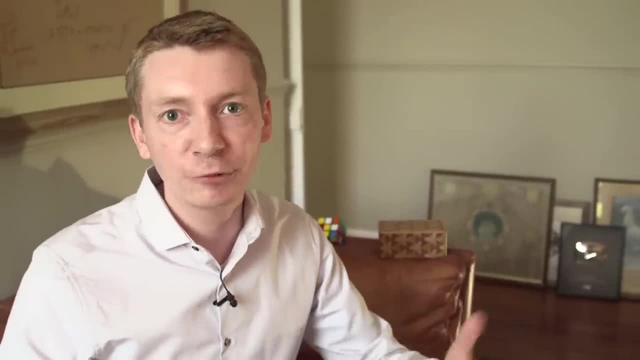 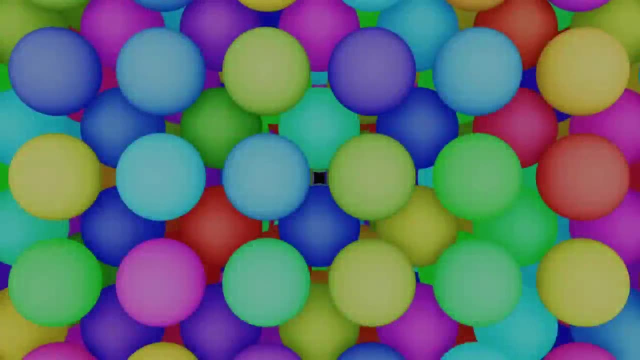 be a bit hand waving, but we're going to try our best. So imagine a sphere packing in three dimensional space. It's going on infinitely. and imagine it's as full as possible as well. So there aren't gaps that are big enough to fit any extra spheres in. So this is as full as possible. 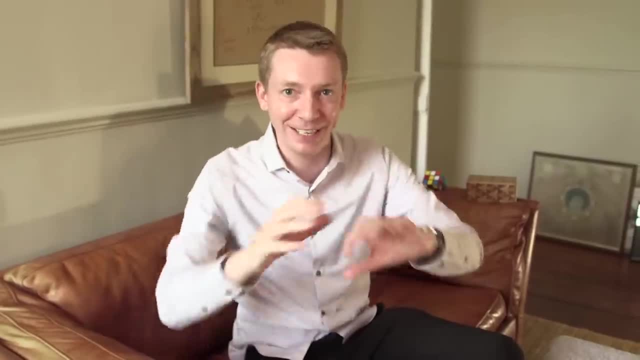 But here's the idea. So you have a sphere, you have a set of spheres, and then you've got a set of spheres. You've got the whole set of spheres, You've got the whole set of spheres. So you've got the. 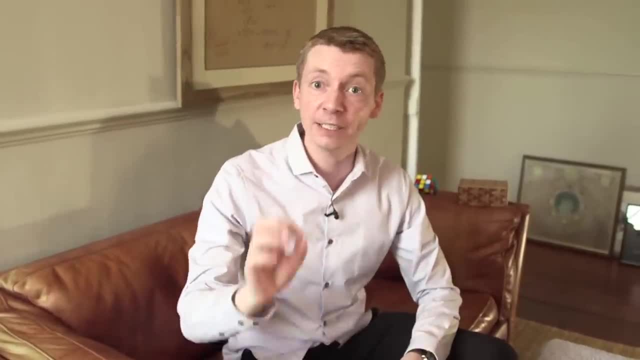 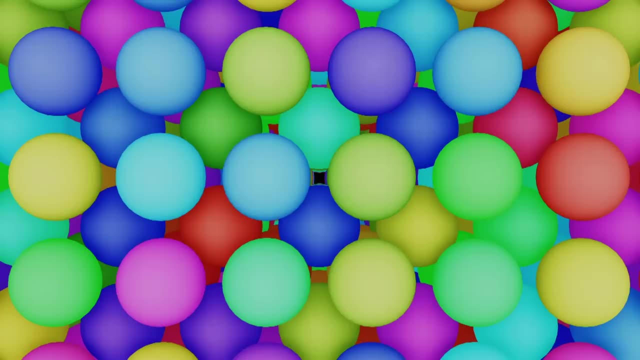 possible. Now. each sphere is defined by its centre, So instead of a problem of packing spheres, you can think of it as a problem of points in space, So like a network of points in space. If each sphere had a radius of one, then these points would have to be. 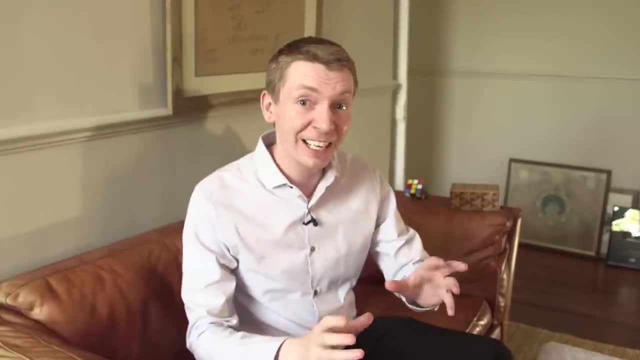 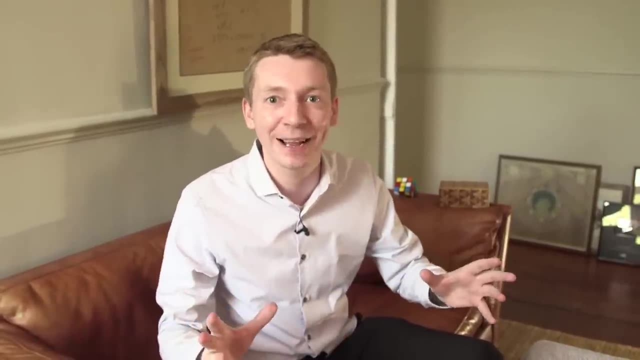 at least two units apart. So what they did is they started looking at the local structure near a given sphere. I'll show you the sort of thing. I mean, If we had, say, one of the hexagonal packings, Let's do that. Let's say we have this centre sphere, here The local. 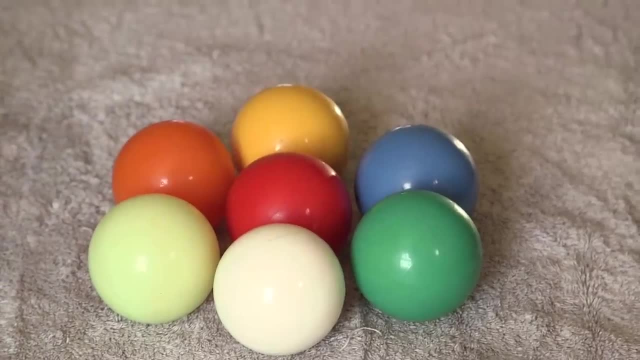 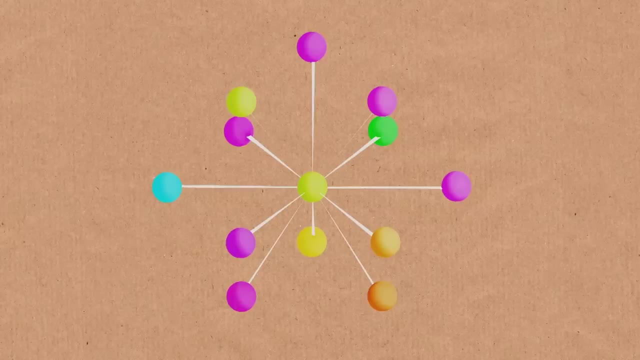 structure to. that would be these six spheres going around the equator. There would be three spheres at the top and three spheres below it. So that would be the local structure around that hexagonal packing. Now they would give the local structure a score. Now that's just. 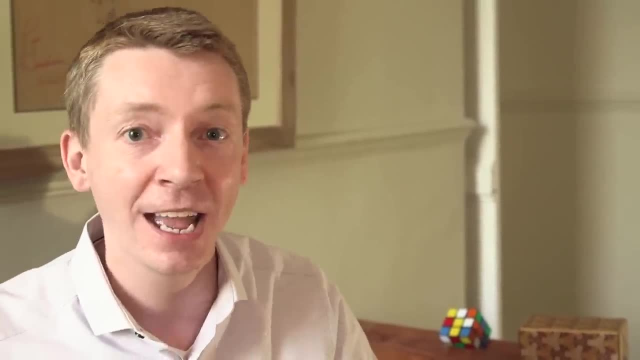 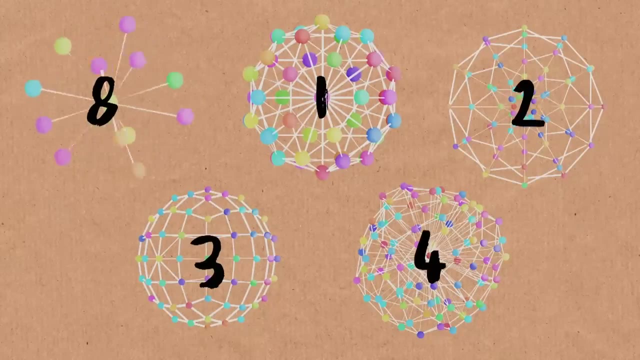 a number. There's a technical definition for that, but they would give it a number. Now, if each local structure has a score less than the hexagonal packing score, then they would have proven the conjecture. So that means that the hexagonal packing would be the densest. 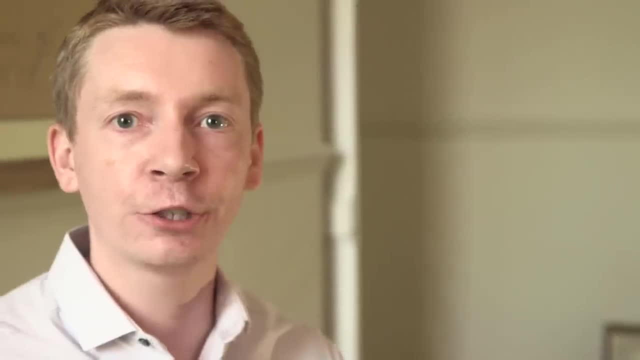 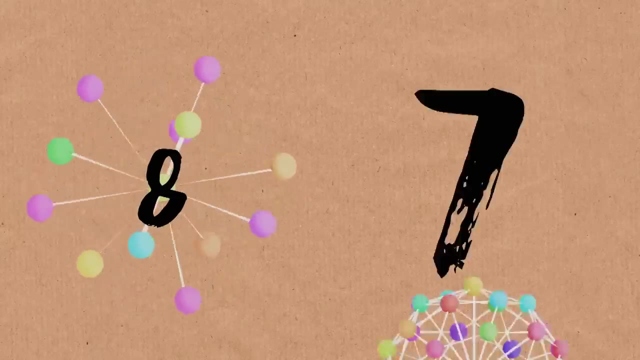 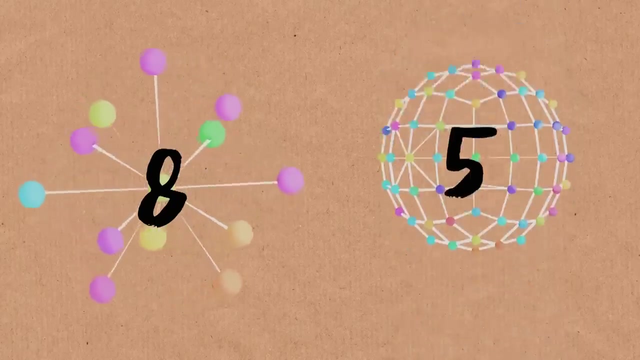 packing. So now the question was: is there a local structure that has a score greater than the hexagonal packing? Is there a counterexample? So what they did is they created a list of 5,000 potential counterexamples. Eventually, they actually whittled that down a bit to. 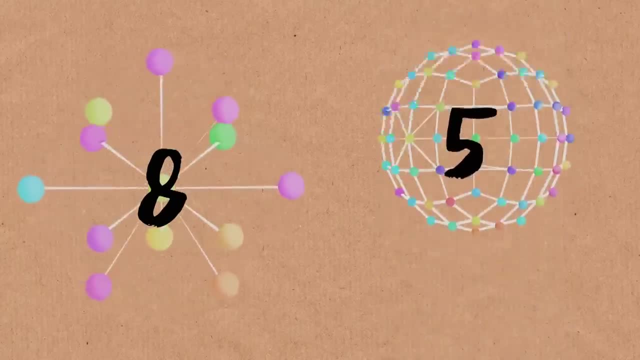 about 100.. And then they just checked them. They just checked them one at a time to see the score, And if each one has a score less than the hexagonal packing score, then they would have a score greater than the hexagonal packing score. So this is a counter-example. 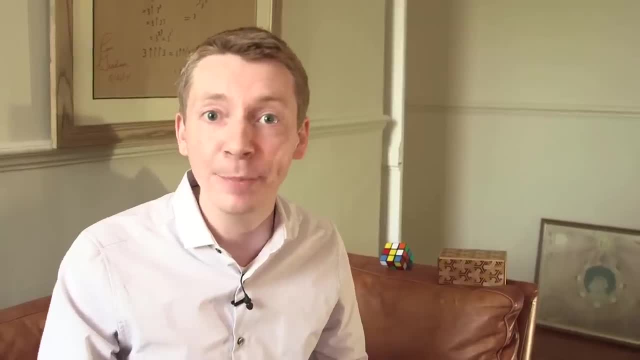 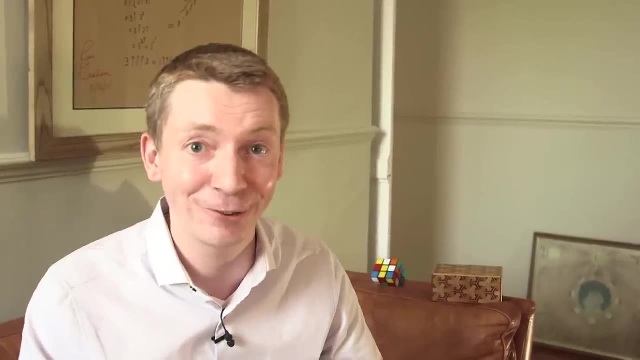 If each one has a score less than the hexagonal packing, you can dismiss it And eventually they were able to dismiss all of 100 of these potential counterexamples, which means there are no counterexamples and that proves the conjecture That means that the hexagonal 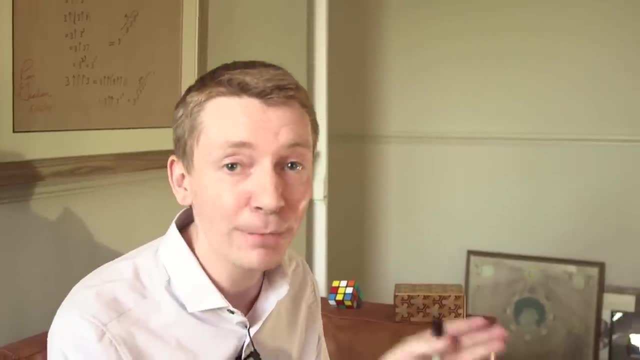 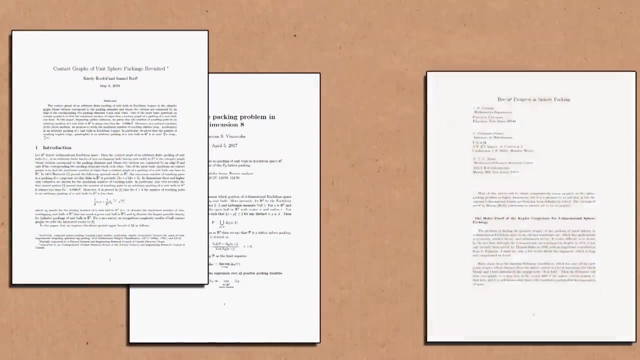 packing is indeed the densest packing possible, at 74.05%, And it was a series of papers throughout the 90s and the theoretical stuff is traditional mathematics. And then, when they started checking through these counterexamples, that was the result. 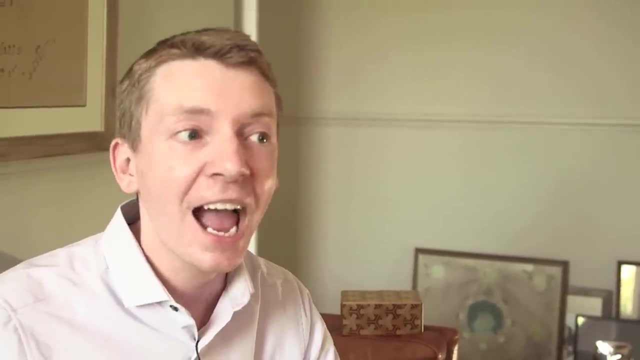 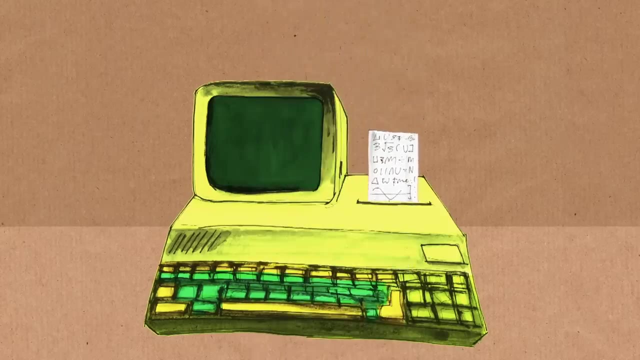 For example. this is what was done by a computer, and this is why they were slightly unsure if the proof was 100% correct, Because you can't check the computer's working really. So that's why they started this project, this 15 year project. it turned out to be: